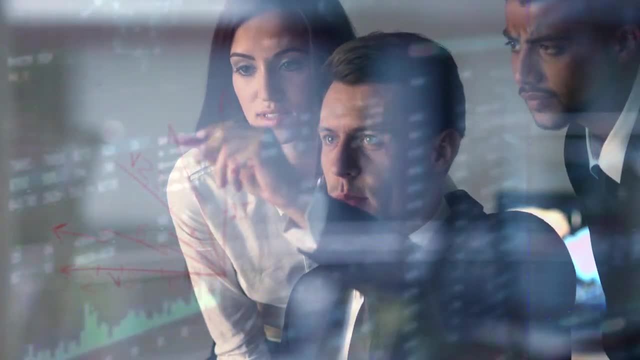 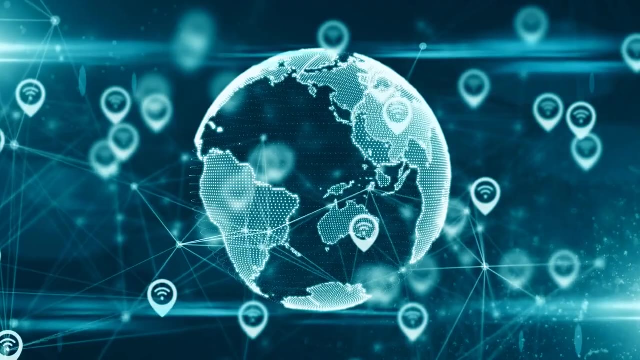 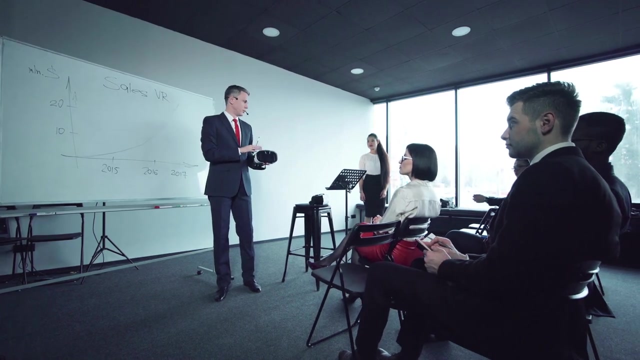 They create models and simulations to help solve organizational problems. They validate and these models with various inputs and parameters. after the model or simulation is created, it gets refined over time as needed operations. research analysts also educate users on how to use the model or simulation that they have created. often they are using sophisticated computer software. 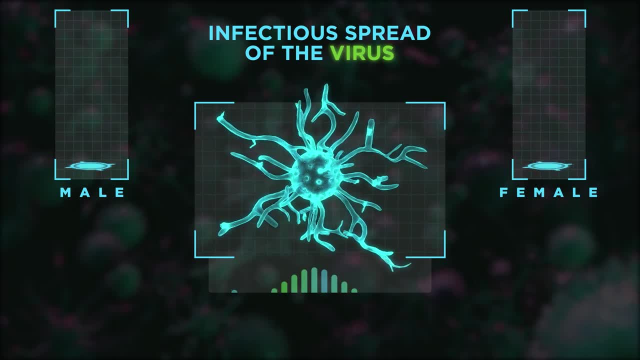 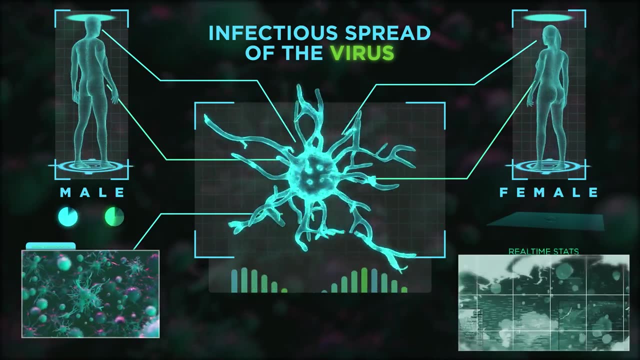 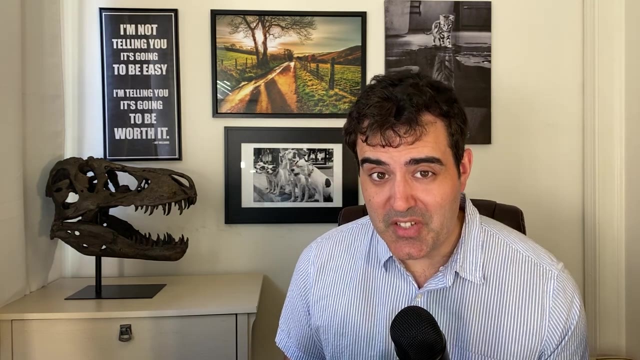 to analyze and build these models. operations research analysts can work for a variety of different organizations. we'll get into the types of organizations a little bit later in the video. so what is the average base salary of an operations research analyst? well, this first set of data is going to be from the bureau of labor statistics. it doesn't include overtime. 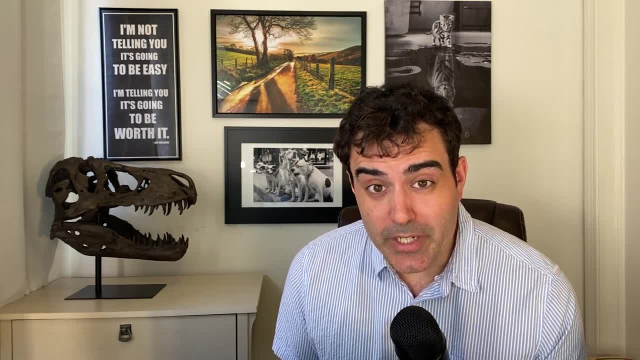 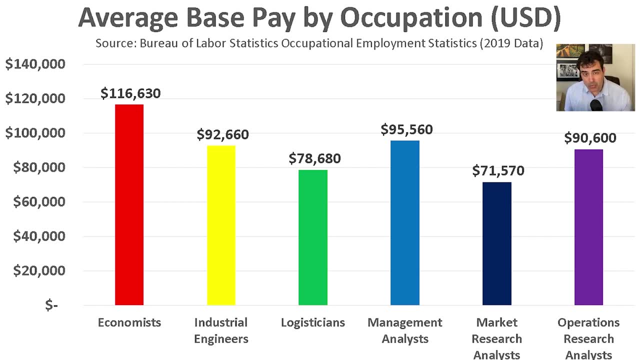 and other benefits. it is only base salaries for employed operations research analysts they do fairly well. their average base salary is a little bit more than logisticians and market research analysts. operations research analysts don't quite make as much as management analysts, industrial engineers and economists, but when you do look at the wage growth over the past 20 years, 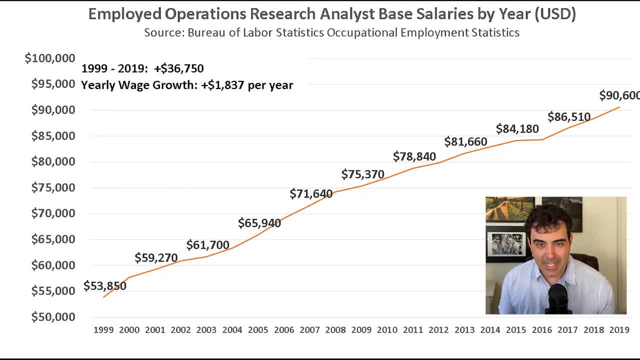 things are going to be a little bit different than the average base salary of an operations research analyst look pretty good for this occupation. in 1999, the average base salary for someone in this occupation was 53 850 dollars. wages steadily rose over the next two decades and then in 2019. the average 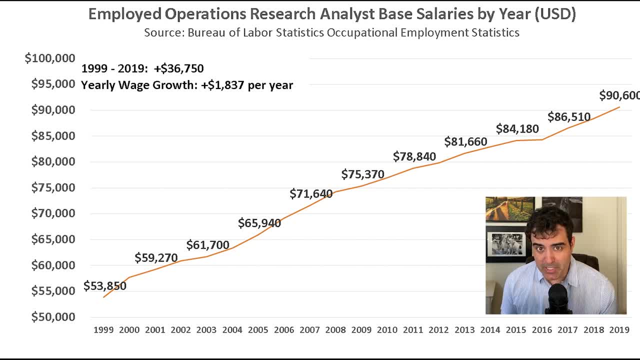 base salary was recorded at 90 600. the new data for 2020 will be coming out in april of this year. so wages rose from 1989 to 2019 by around 37 000, which gives us an average yearly wage growth of about eighteen hundred dollars per year for this occupation. if we were to forecast this into 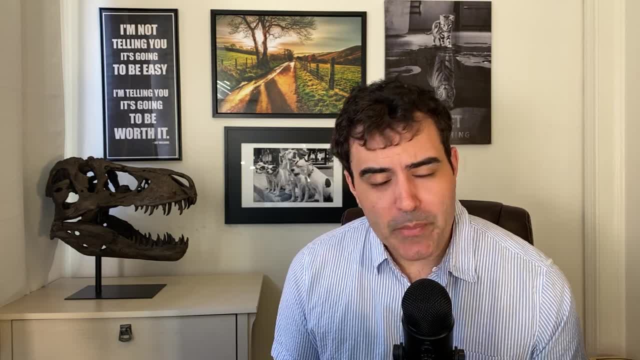 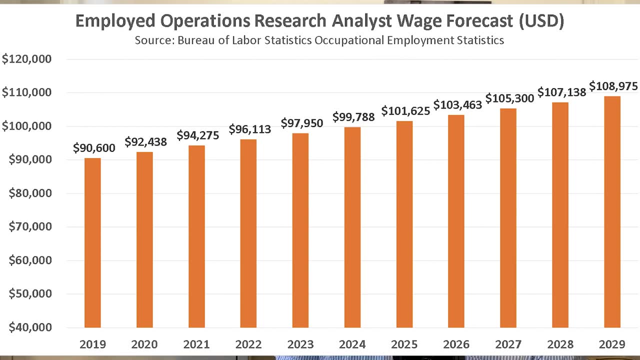 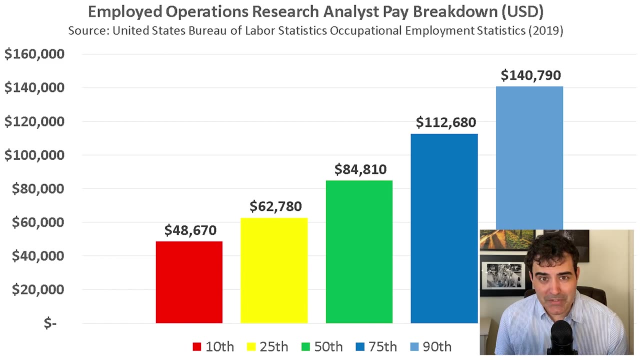 the future. the average base salary in 2021 would be around ninety four thousand dollars, and then, by 2029, wages should rise to around 109 000 per year as an average base salary. experience plays a huge role in this occupation, a starting salary meaning probably around the 10th percentile among 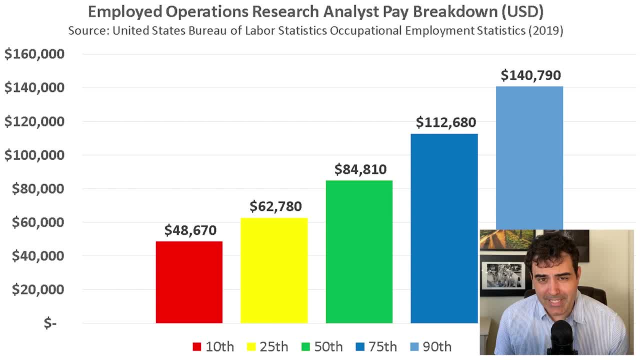 all operations, research analysts would be around forty nine thousand dollars per day year, Whereas someone that's really late into their career and lives in a hot job market. the top 10% of operations research analysts start at around $141,000, and then they go up. 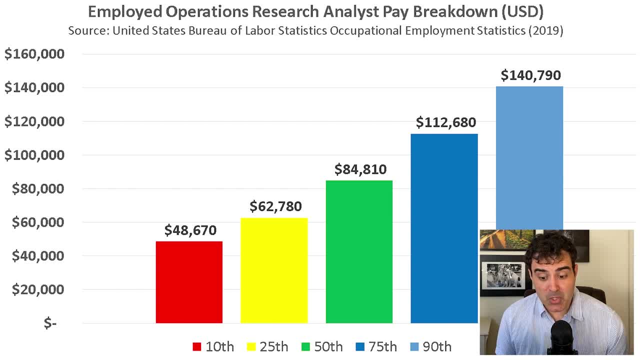 from there. So there is a $92,000 difference between a starting salary for someone in this occupation and someone that's really late into their career and works in a hot job market and probably a hot industry as well. Geography is one of the variables that influences the compensation. 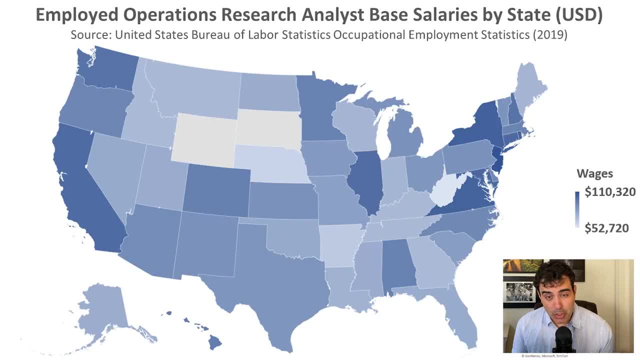 of operations research analysts. In this map, the dark blue areas are the high paying states for this occupation, and the lighter blue areas pay less. As for the beige colored states, there's actually no data for those two states in this map, So the lowest paying state is the state. 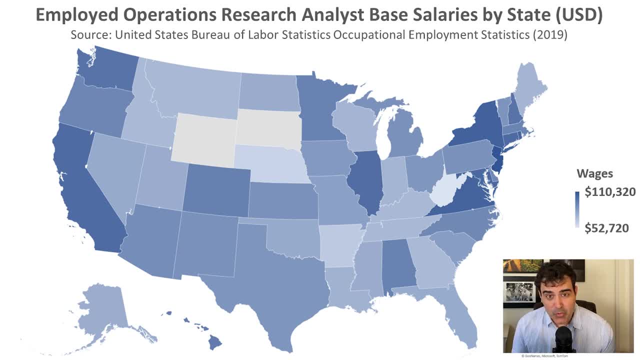 of West Virginia, with an average base salary of around $53,000 per year, Whereas the highest paying state- interestingly, it's not New York, It is actually New Jersey, where the average base salary for an operation is $53,000 per year. So the lowest paying state is the state of West. 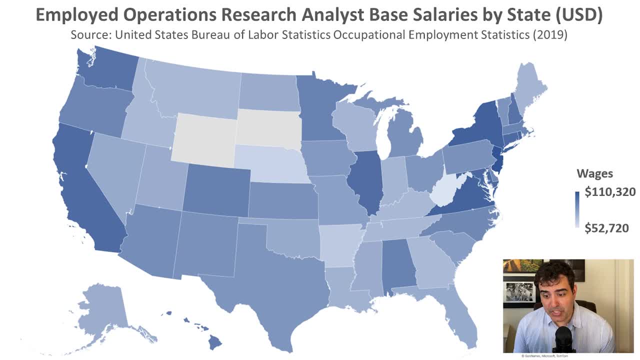 Virginia and the average base salary of someone working in New Jersey. Other high paying states include the Washington DC, which isn't a state, but it's included here anyways- the state of New York, Virginia, Rhode Island, Maryland and the state of Connecticut. Like I said before in this, 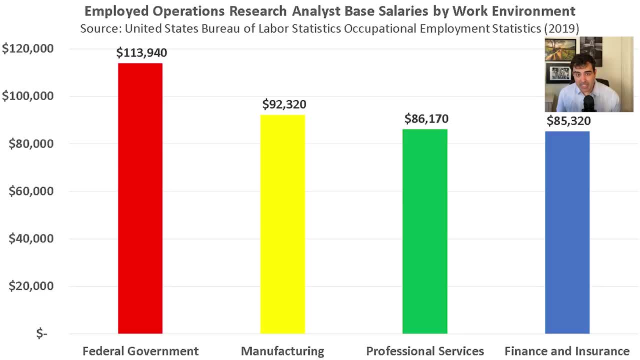 occupation industry matters. So the lowest paying state is the state of West Virginia, where the average base salary of someone working in New Jersey matters. The federal government pays operations research analysts on average the greatest amount of money. The average base salary for someone working in the federal government is $114,000 per year And the next highest is 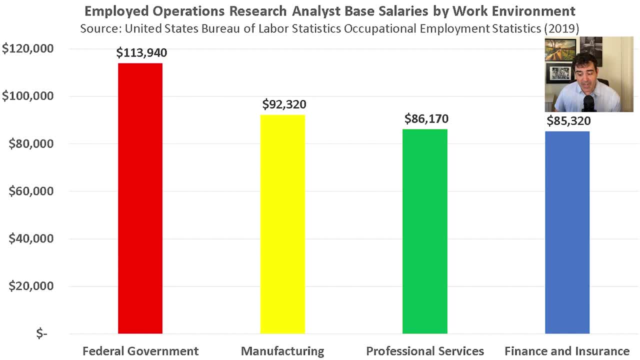 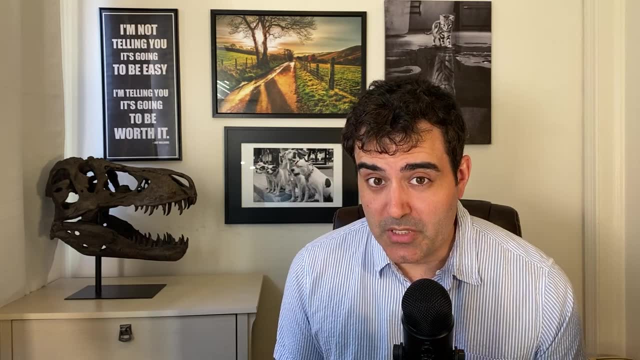 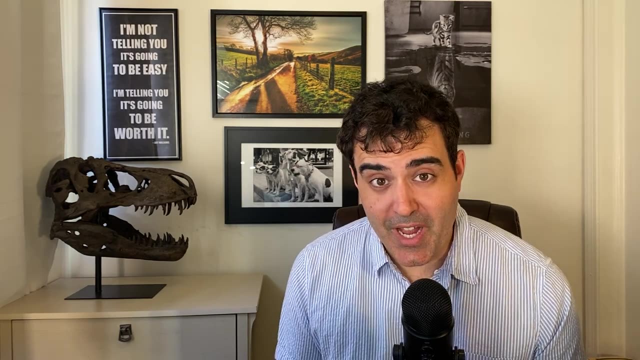 the manufacturing industry, and then professional services And finally finance and insurance. A lot of the federal government jobs support the department of defense, and many of them are in the Washington DC metro area. So what is the job market like for this occupation? Is it a growing field, or is it a shrinking field? And how hard is it to get? 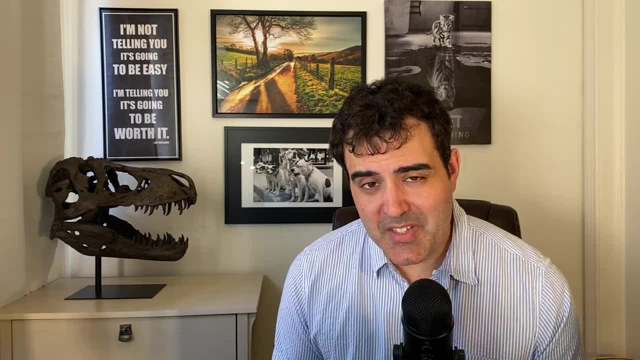 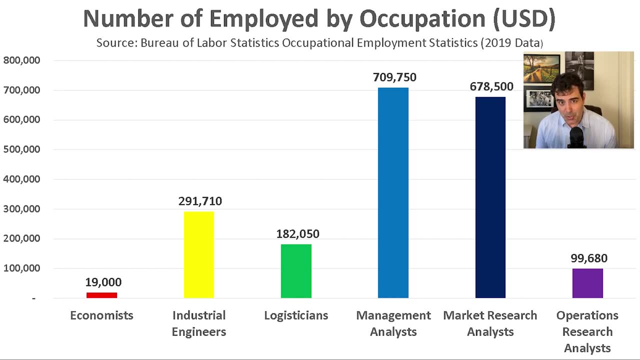 a job in this occupation. Well, the first thing to keep in mind is this is a moderate sized occupation. There's about a hundred thousand employed operations research analysts across the country. This is much more than economists, but this is much less than management analysts. 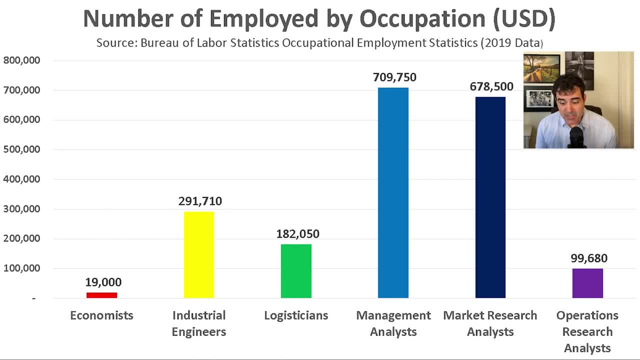 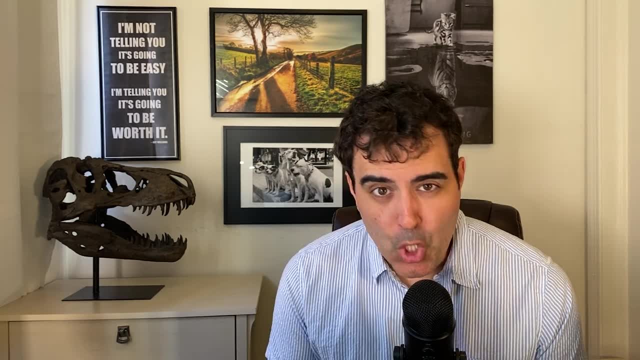 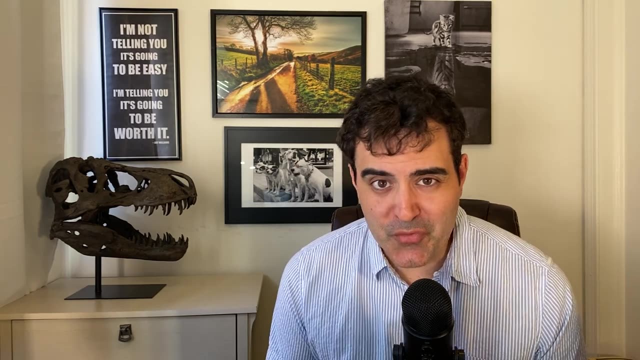 market research analysts, and this is less than industrial engineers and logisticians. So the workforce for this occupation is moderately sized. With occupations that have smaller workforces, sometimes you have to move across state lines in order to get the best job opportunities, But things are changing for this occupation. 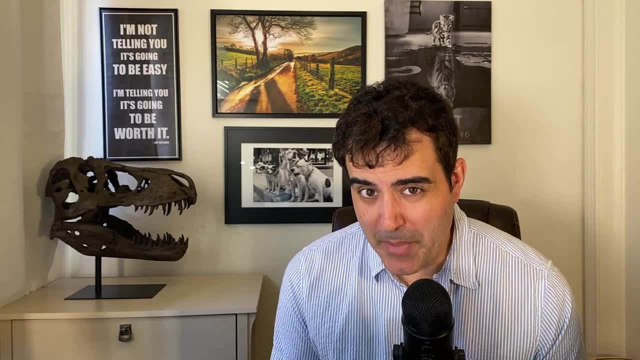 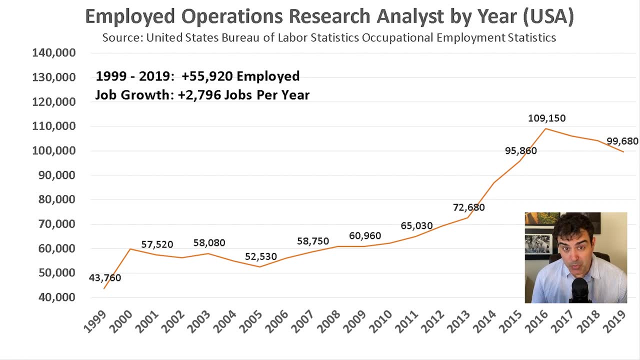 There has been definitely a growth in the number of jobs over the past two decades. In 1999, there was about 43,760 employed operations research analysts across the United States. By 2019, this rose to 99,680 employed operations research analysts. 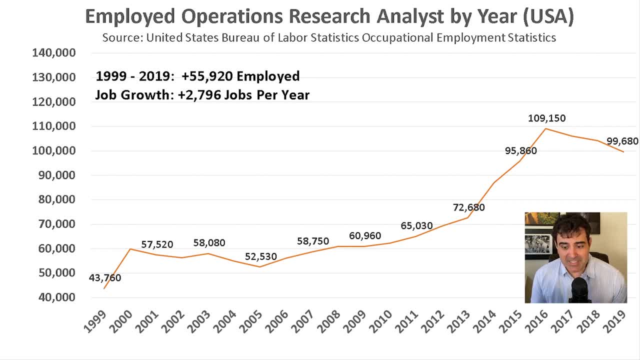 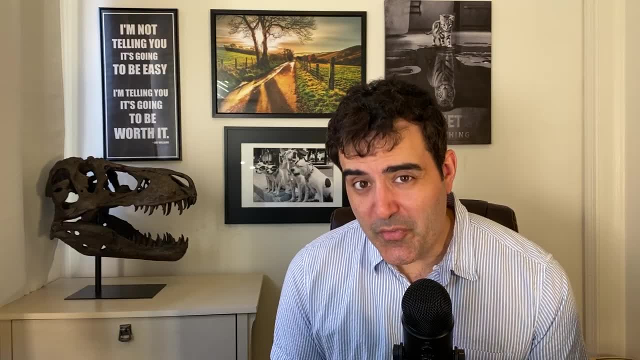 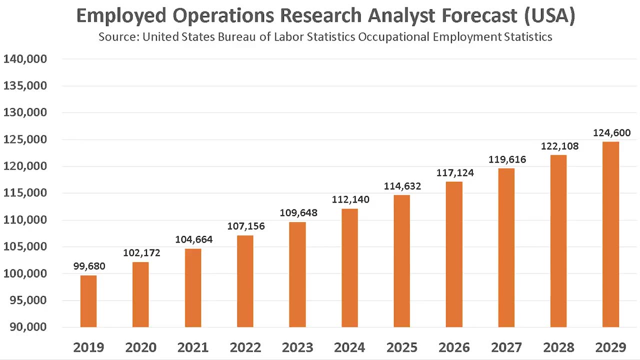 across the country. So, from 1999 to 2019, the number of people in this occupation has more than doubled. Not only that, the federal government is predicting a 25% increase in operations research analysts over the next 10 years. This means that by 2021, they're projecting around 105,000 in the occupation and by 2029, about 125,000.. To put this into context, the average occupations workforce is only expected to rise by 4%, whereas the average occupations workforce is only expected to rise by 25%. But definitely one thing to keep in mind is that this is a very regional occupation and 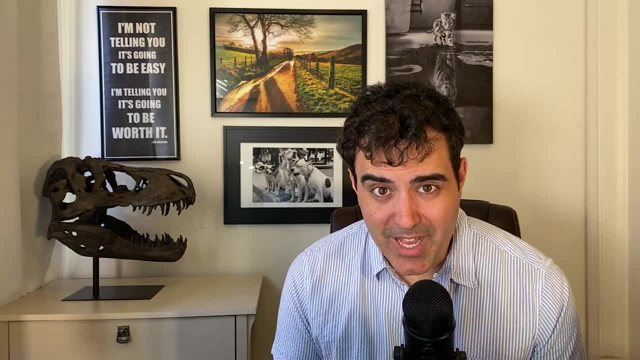 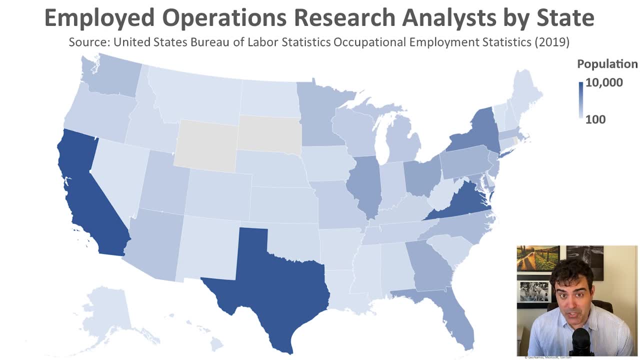 this happens a lot with operations that are moderately sized. The state of California, Texas, Virginia and New York tend to have the greatest number of employed operations. research analysts. This is where a lot of the opportunity is in this occupation And this happens a lot with moderately sized occupations. They might have regional hubs. 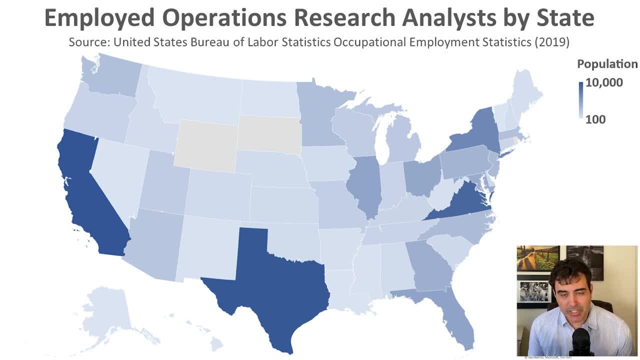 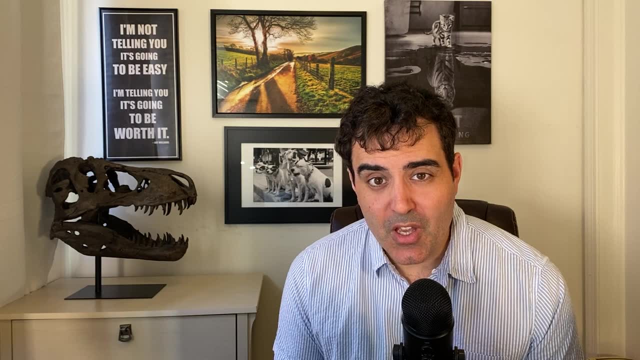 where that's where all the opportunities are, And sometimes to work in this occupation you have to move to one of these areas. Another great metric to look at is the number of job postings right now. When I went on Indeedcom and I searched for operations research analysts across the United. States, I got about 14,500 job openings across the country. Given that there's only about 100,000 employed, this is a lot of job openings compared to the size of the workforce. In fact, this gives us a ratio of one job opening on Indeedcom per seven employed operations. 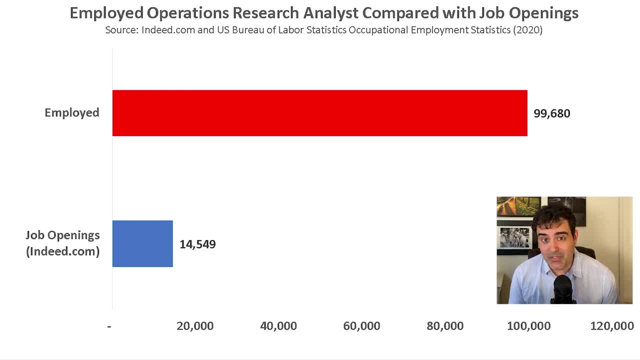 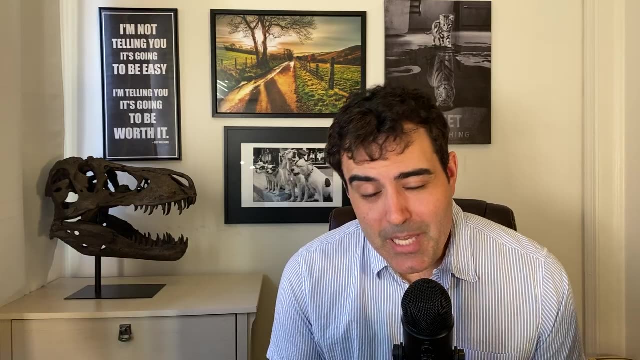 research analysts. Anytime the ratio is less than one to 15, this indicates somewhat of a shortage. So right now, based off the number of job postings across the country, this indicates that there is a shortage of people in this occupation. Now, like I said previously, people in this occupation can work in a wide variety of different 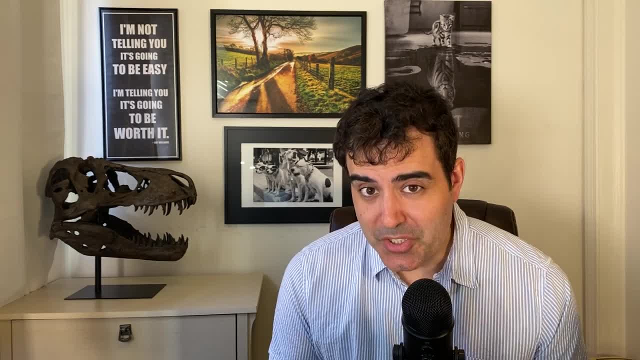 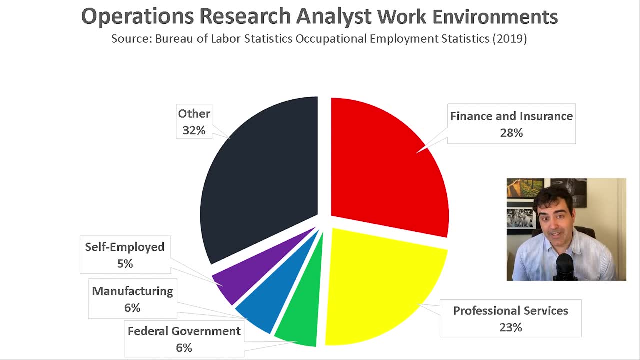 industries: 28% work in the finance and insurance industry, 23% work in professional services. only 6% work in the federal government And, again, this is the most lucrative industry for people in this occupation- the federal government. About 6% work in manufacturing and about 5% are self-employed. 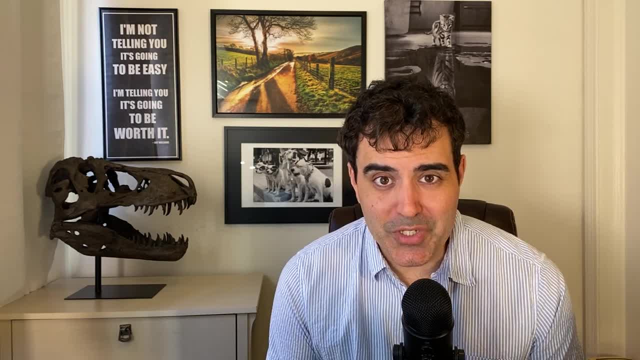 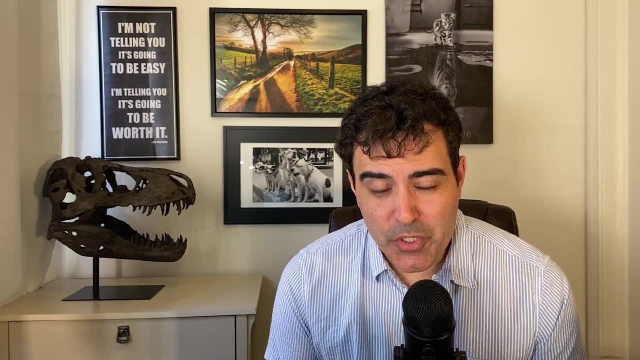 So the next question is: would this occupation be compatible with your interests? To determine this, definitely look into taking a RIASEC assessment. A RIASEC assessment is an interest inventory. You fill out a free assessment online. There's quite a few available all across the internet. 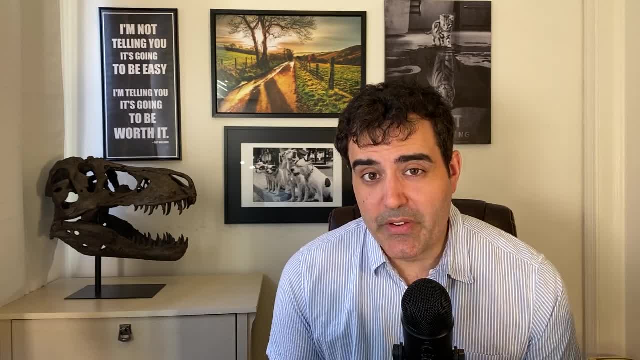 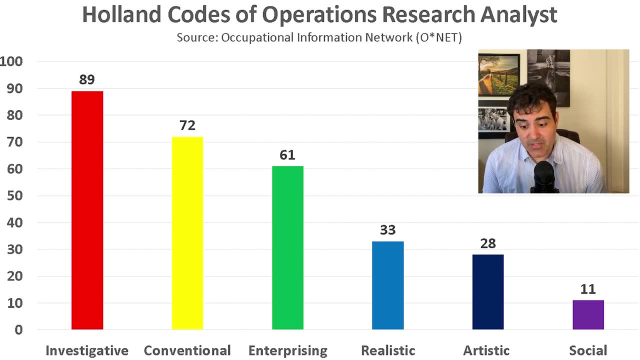 At the end of the assessment it gives you results scores for six different themes: Operations research analysts that take the RIASEC assessment tend to score high in the investigative, conventional and enterprising themes. People that score high in the investigative theme tend to be a little bit more introspective. 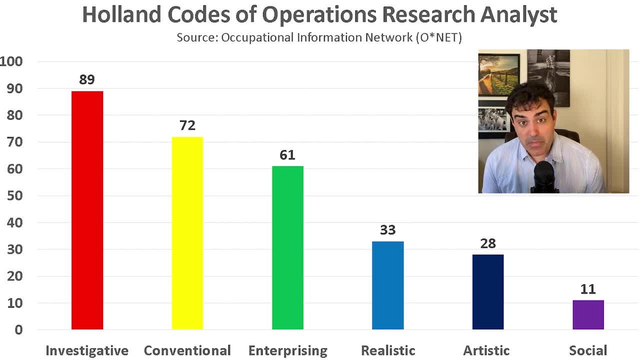 They like learning new things and they tend to be pretty curious people. People that score high in the conventional theme: they hate chaos, They love organizing. They like organizing data and other information into systems that can be easily understood. And people that score high in the enterprising theme tend to like leading people and they 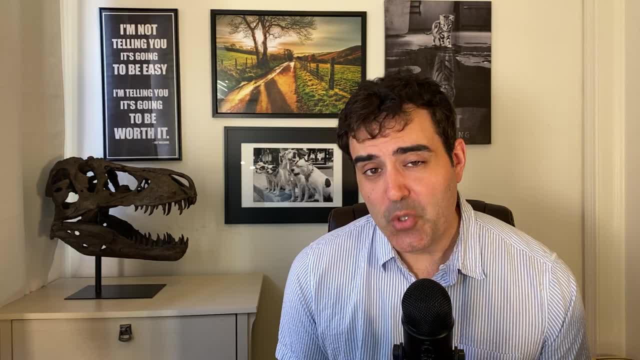 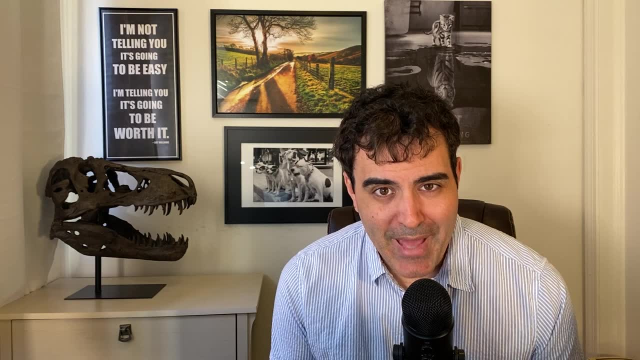 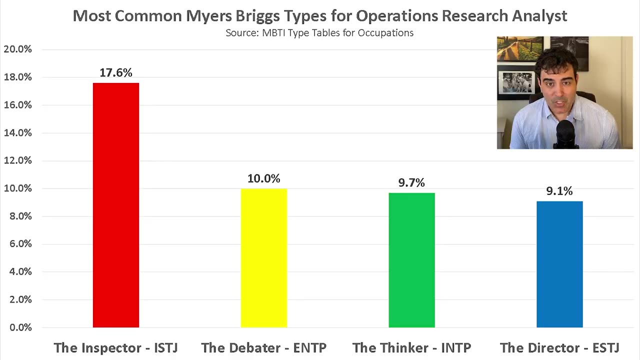 can be somewhat entrepreneurial as well. So if you also take a RIASEC assessment and you score high in these three themes, this could indicate that this occupation might be compatible with your interests. Another data point is: would this occupation be compatible with your personality? 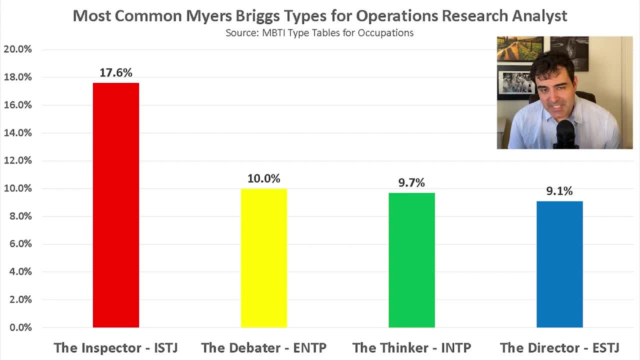 According to the Myers-Briggs company, they found that 8% work in manufacturing and other information into systems that can be easily understood. 18% of people that work in this occupation are ISTJs. 10% are ENTPs. the debater about 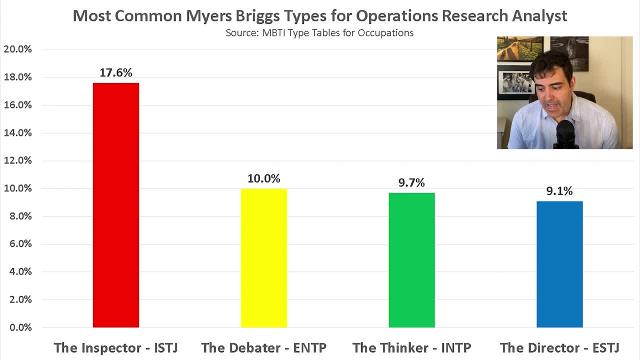 10% are also INTPs- the thinker- and about 9% are ESTJs- the director. Notice that all four Myers-Briggs type. they have a preference for thinking over feeling. Finally, what is required to become an operations research analyst? 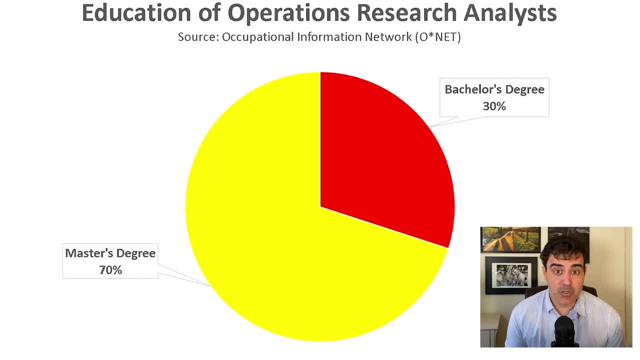 About 30% of people in the occupation, according to the Occupational Information Network, have a bachelor's degree, whereas the vast majority of people in this occupation have a master's degree. So to get the better jobs in this occupation, you might need to get a master's degree. So, as you can see, there are pros and cons to becoming an operations research analyst in 2021.. Operations research analysts do make a pretty good amount of money. They don't make quite as much as economists, but they do make more than many other similar. occupations. One of the greatest advantages of this occupation is that they have the ability to work in a job market. The workforce in this occupation has doubled in 20 years. The government is anticipating a 25% growth in the workforce over the next 10 years. 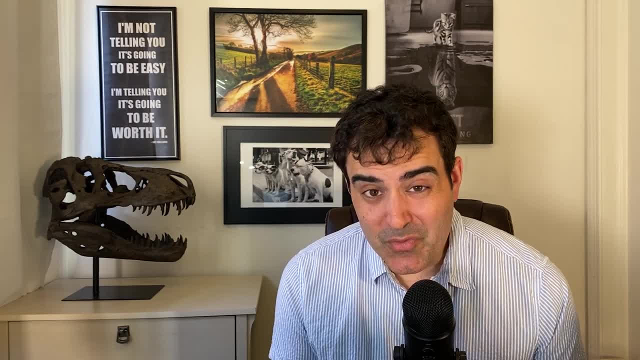 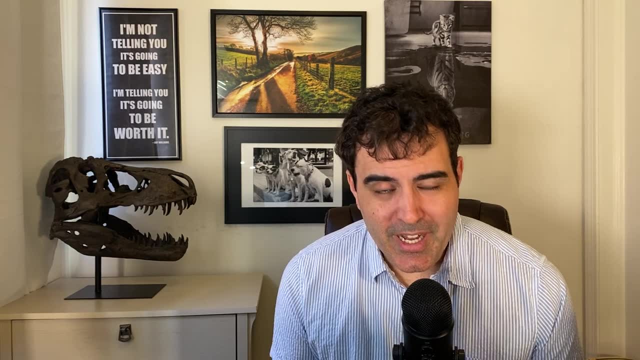 And based off the number of job postings around the country, there's definitely a shortage of operations research analysts in many different states and metro areas. It is always great to be in an occupation that has such high demand. Education is a barrier to entry.